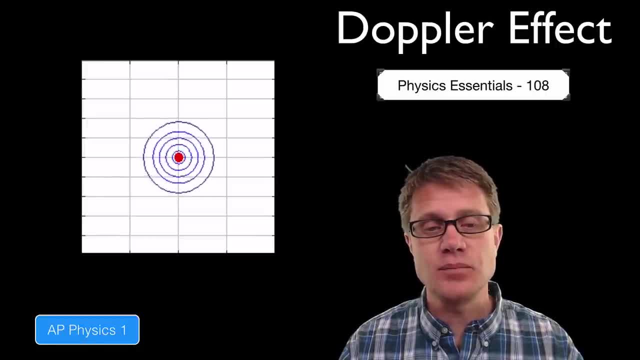 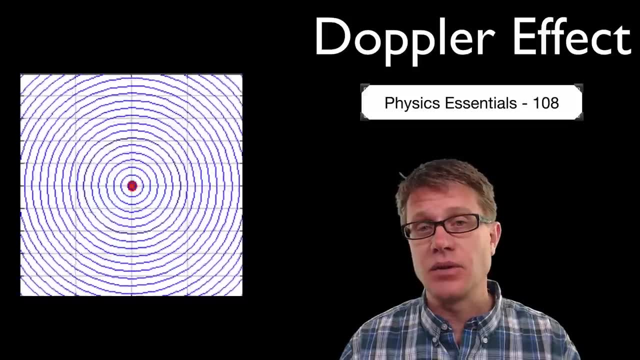 occur if you are moving, And we will get into that in just a second. So let's say, this point here is generating sound waves. They are moving away from that point, And so if you were to listen to them, those sound waves would be hitting you at the same rate, and so it would. 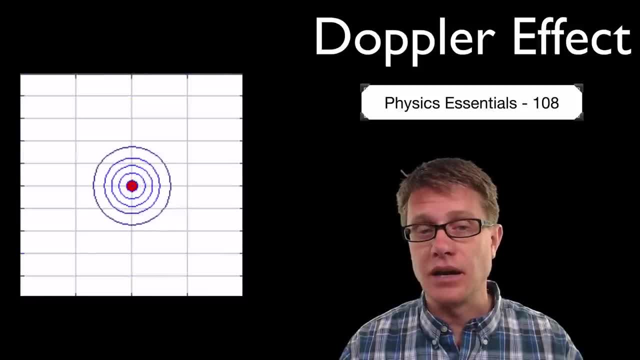 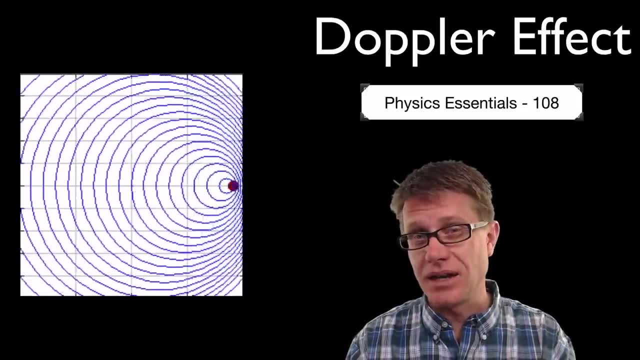 be a constant pitch, But watch what happens if we move that object from left to right. As it moves from left to right, you can see that the waves in front of it are bunching up. What would that sound like? An increase in pitch? And then behind it, they are actually. 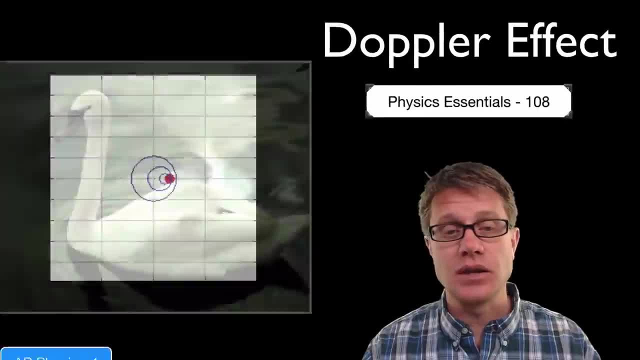 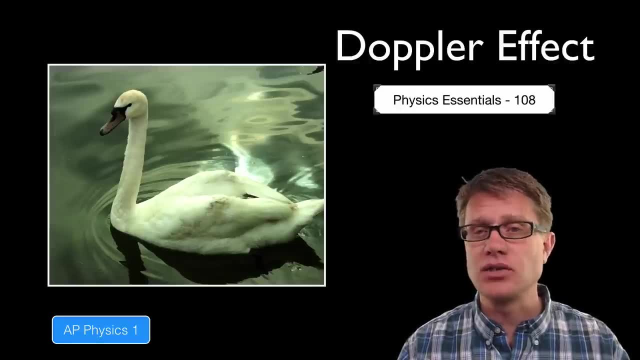 spreading out, We would hear a decrease in pitch. You could see the same thing in water waves. This swan, we know, is swimming from right to left. It is swimming to the left. How do we know that? Well, it is generating water waves And the 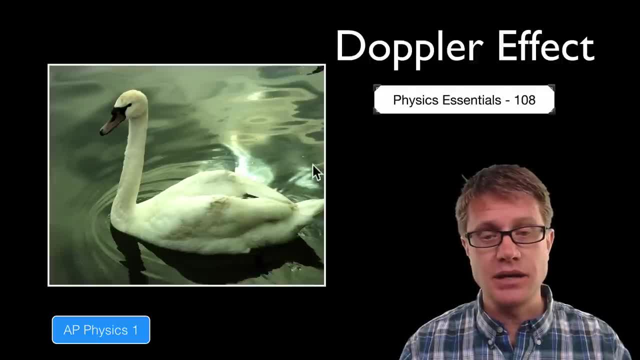 one that is swimming from the left to the right is the one that is generating the sound waves And the one that is in front of it, you could see, are getting bunched up And the ones behind it are actually spreading out. So that tells us it is moving to the left. It also has its beak pointed. 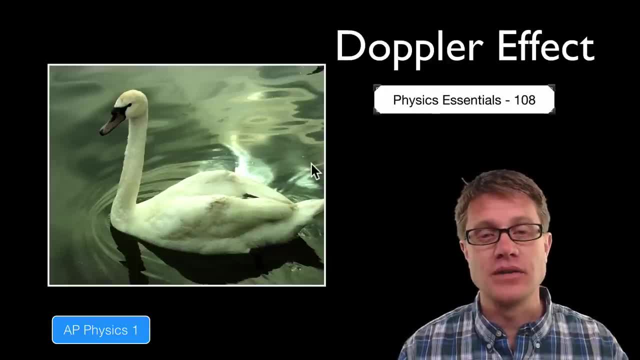 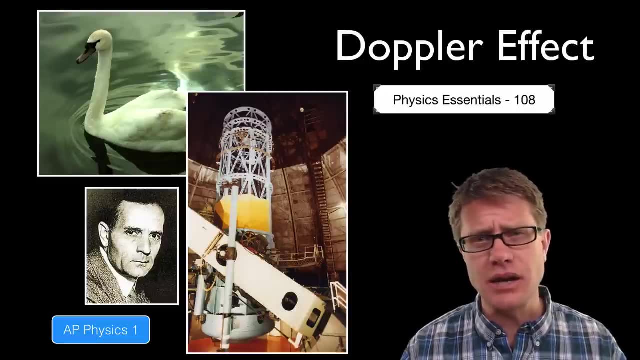 in that direction as well. Now it is not only sound and water waves, but light is going to do the same thing, And one of the greatest discoveries ever was Edwin Hubble's discovery that wherever he looked out in space, all light seemed to be shifted to the red. We call that. 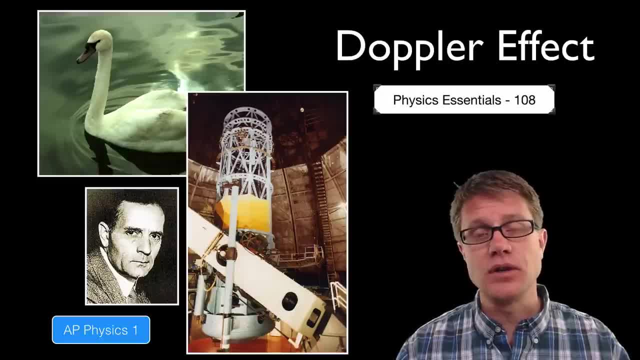 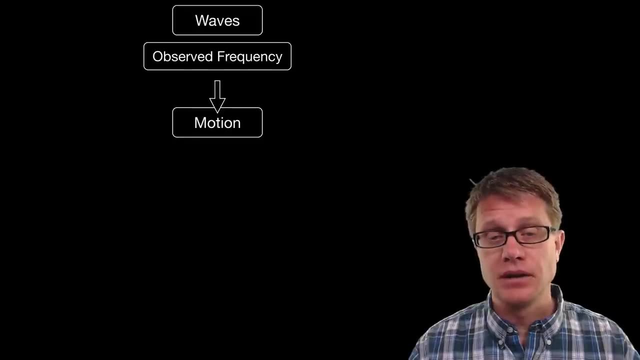 a red shift. What did that mean? All the light that he saw was moving away from us, And that indicated we were living in space. We are living in a universe that is constantly expanding, So Doppler effect has these amazing repercussions, And so waves and their observed frequency will change due to motion, And let's 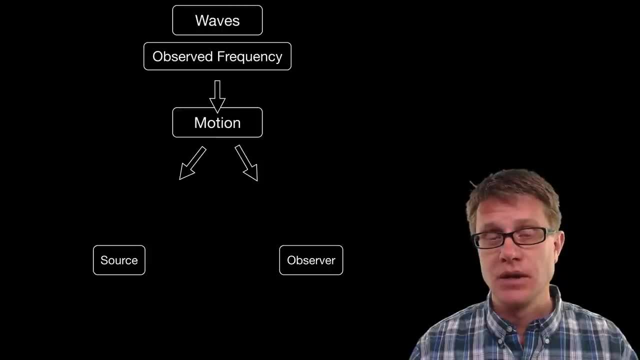 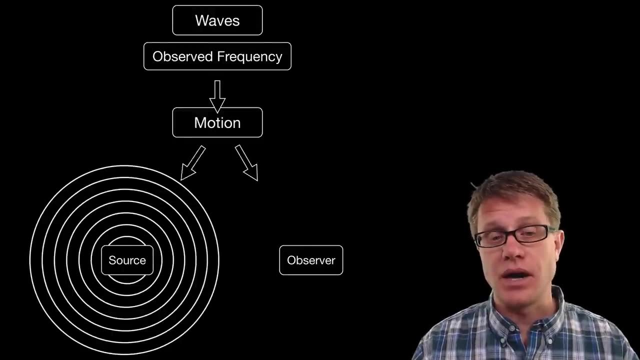 say we have got a source of those waves and then we have got an observer. If the source of the waves is generating waves that move out, they will be of uniform distribution unless it is moving. So as that source moves, as it approaches the observer, we are going. 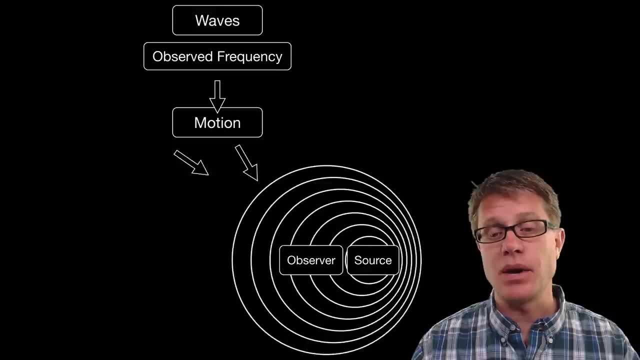 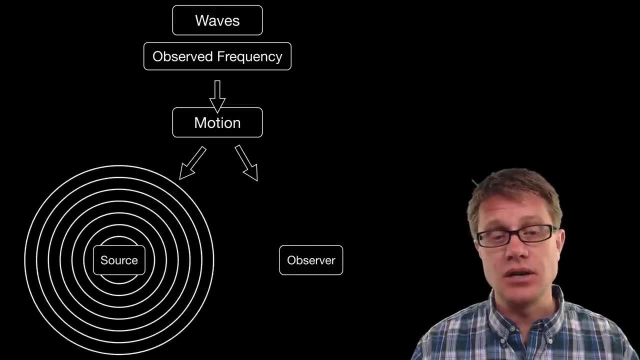 to see an increase in the frequency of those waves, And that is what we are going to be hearing. And then, as it passes the observer, we will see a decrease. But it is not only the movement of the source, It could also be the observer As it approaches the source. 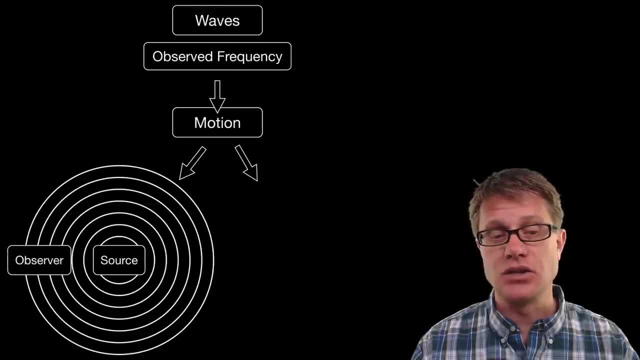 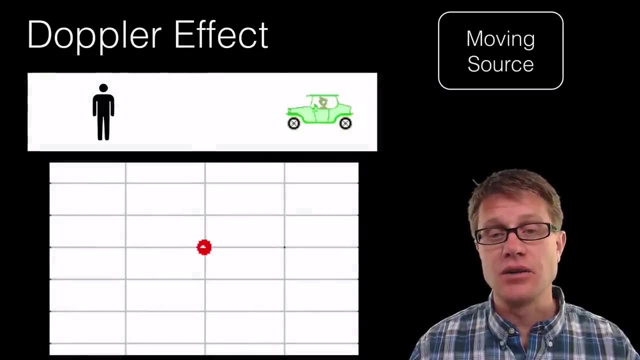 it will hear an increase as it goes towards it, And then there will actually be a decrease as it moves away. And so let's give me a real example of that. Let's say you are standing there and a car is approaching you, The waves, as they come towards you will bunch up And